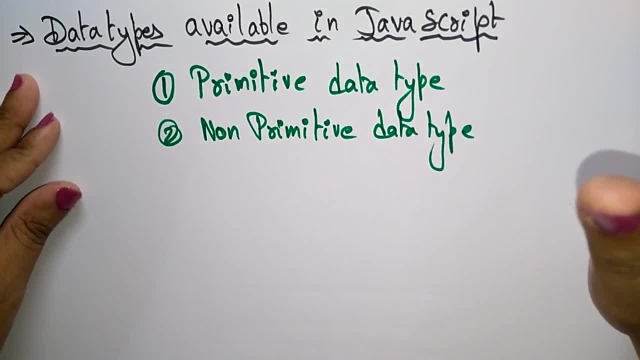 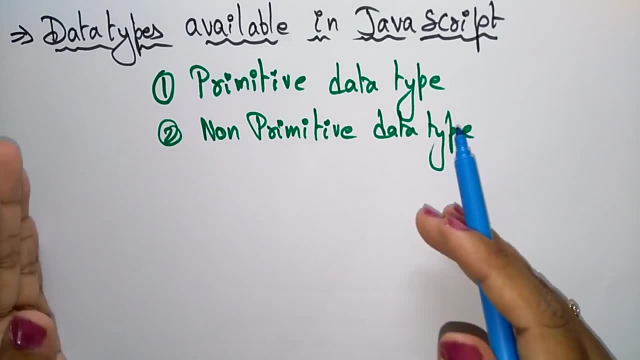 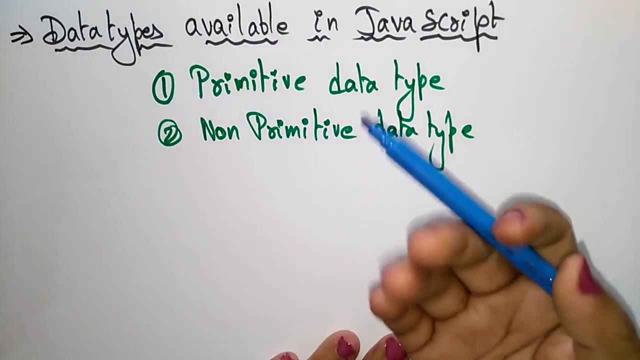 So before going to this topic, Let me explain. just recall that javascript is a dynamic type language. I said it is a dynamic type language, which means you don't need to specify type of variables, So, whereas in the html or in other programming language like the c, whatever the language you are taking, So for that you need to specify the type of variable that you are using. whether you are using the integer or a float or character or string, like that, you need to. 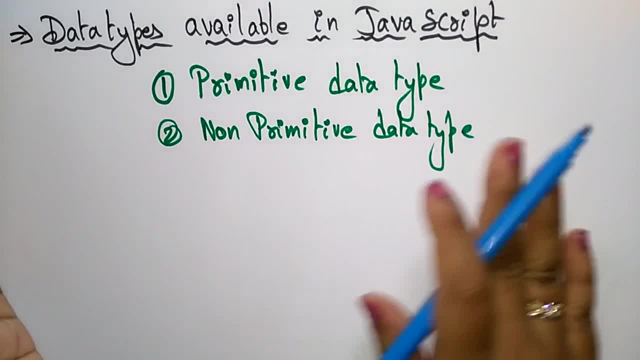 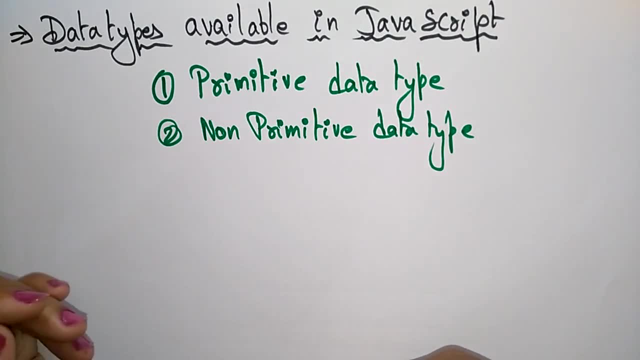 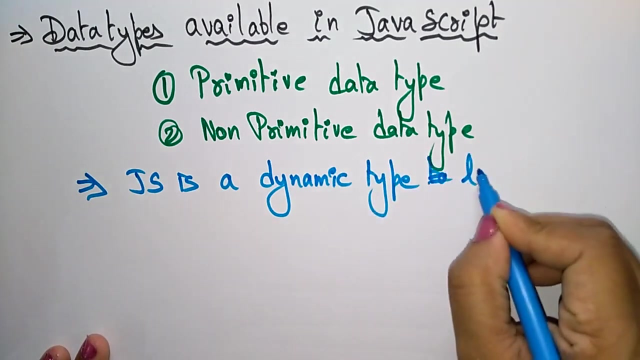 Declared, but in the javascript you no need to specify the type of variable because it is dynamically used by the javascript engine. Let me write that point so that you can refer it easily. Javascript is a dynamic type language. It is a dynamic type language, so for that reason. 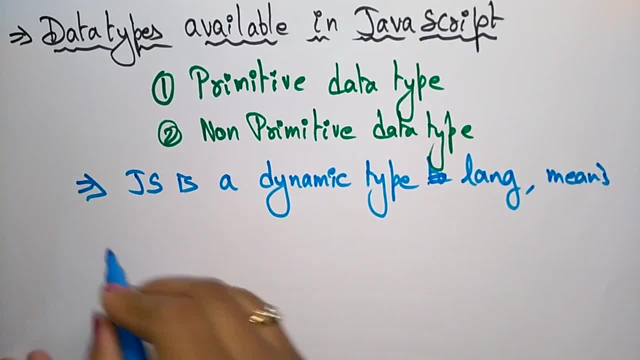 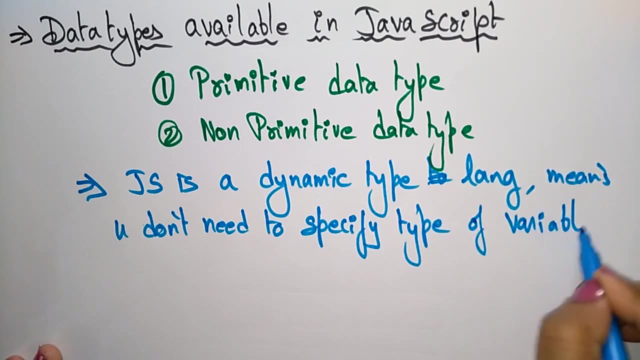 It is a dynamic type language So for that reason Means you don't need to specify. you don't need to specify type of variable. Whatever the type of variable you are using, whether you are using the integer or a character or a string- you don't need to specify. 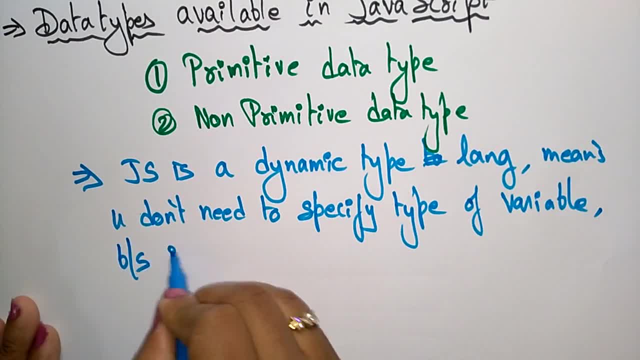 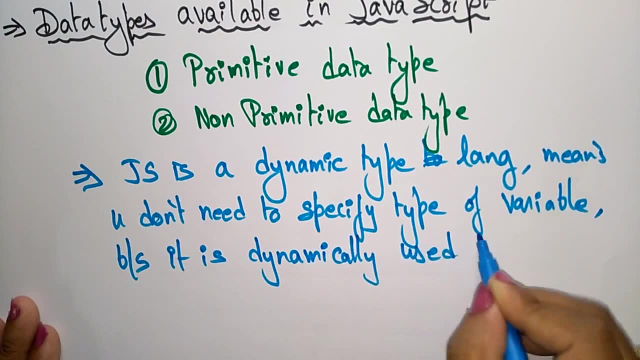 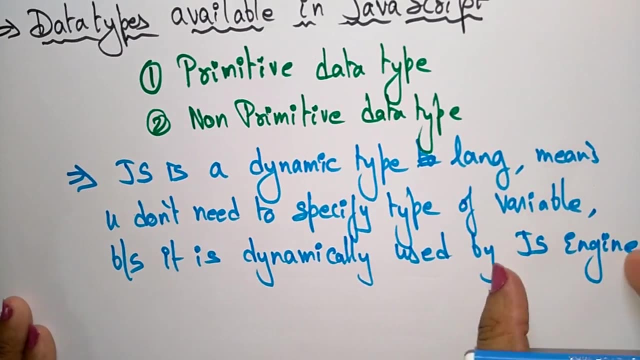 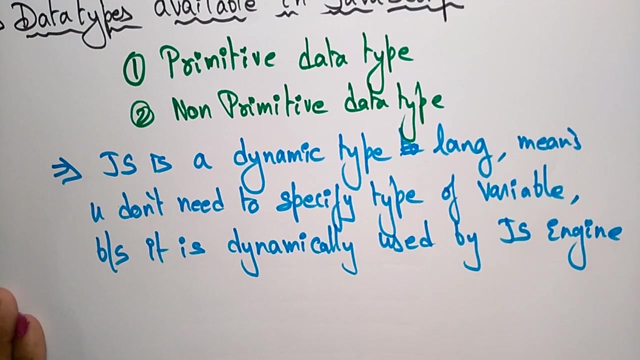 Because it is dynamically, because it is dynamically used by JavaScript engine. So whenever the program is going to be executed, so that dynamically the JavaScript engine is identifying what type of variable you are using in the program, So you don't need to specify that, So you need, just you need to use variable. 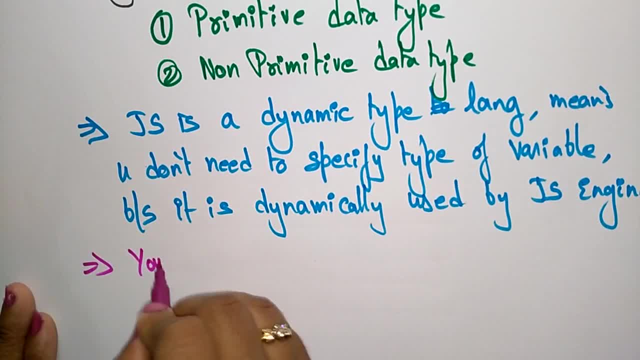 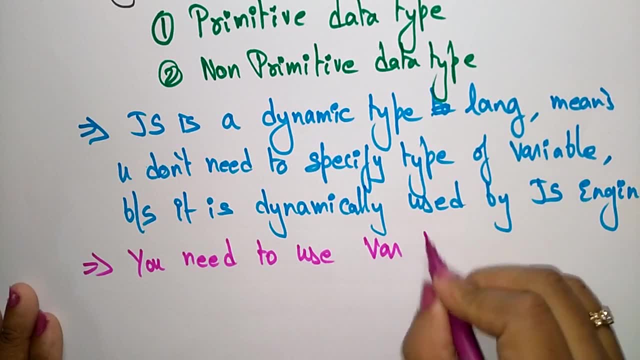 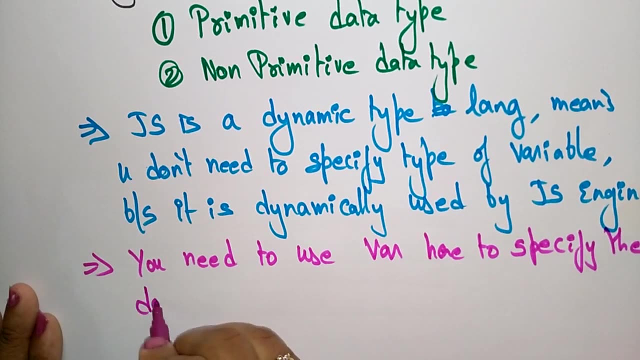 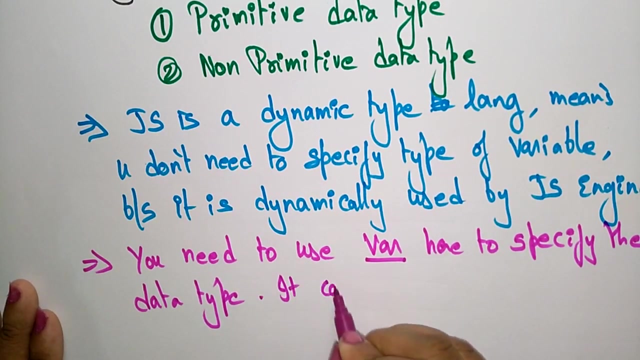 Just use. you need to use var. Var means variable Here to specify the data type. So whatever the data type you are using for that, you just use the name var. It can hold that. var variable can hold any type of var. 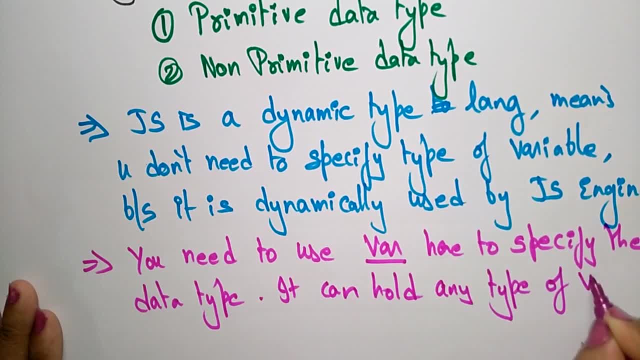 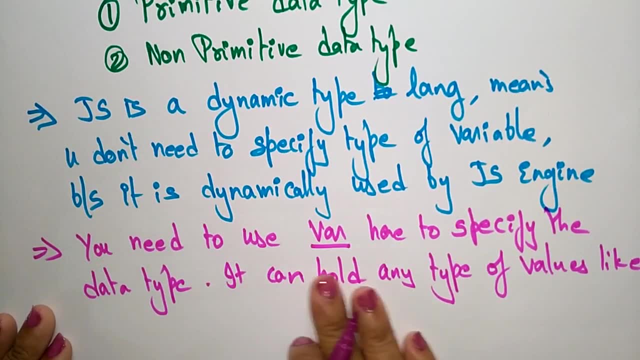 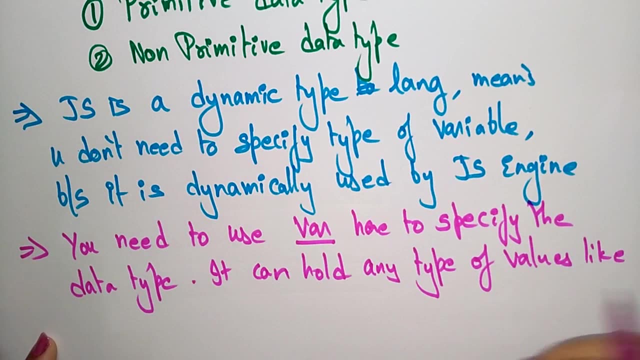 Any type of values like. so let's continue this Here. you need to use var here to specify the data type. It can hold any type of values like numbers, strings or even characters, etc. So the example for this is just: you need to specify. 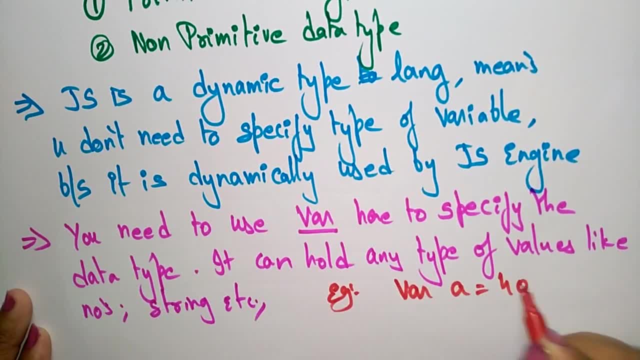 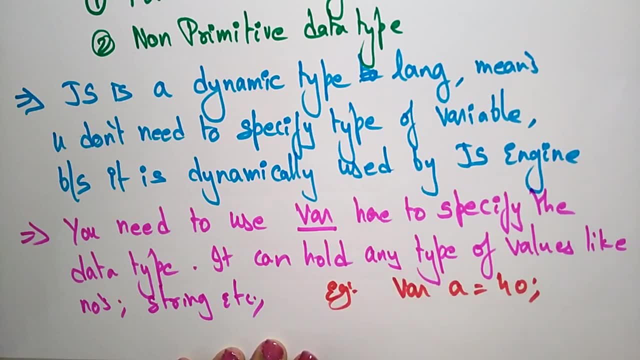 var a is equal to 40. So this is an integer value. I just specifying here var. I am not writing any data type, int, character or whatever it may. I am not specifying because the JavaScript engine automatically detects what type of variable you are using, data type you are using. 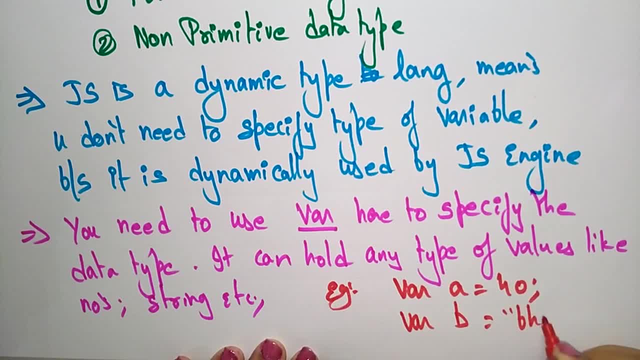 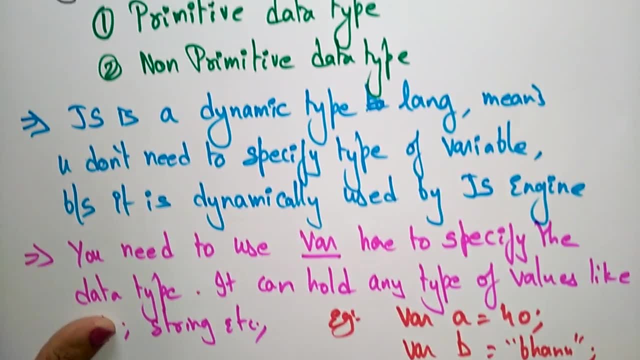 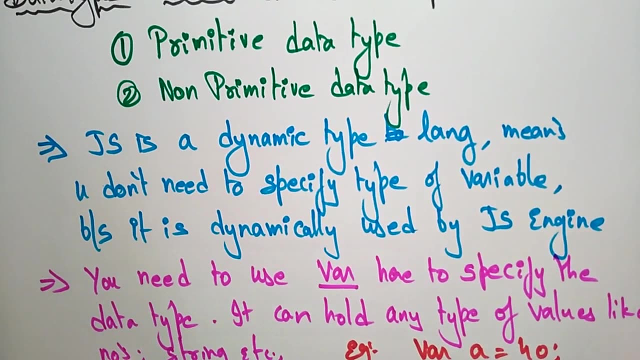 And even you can write: var b is equal to- let's take bhanu. So this is a string. So this is how you are going to use the data types. Because JavaScript is a dynamic type language, you don't need to specify what type of variables you are using. 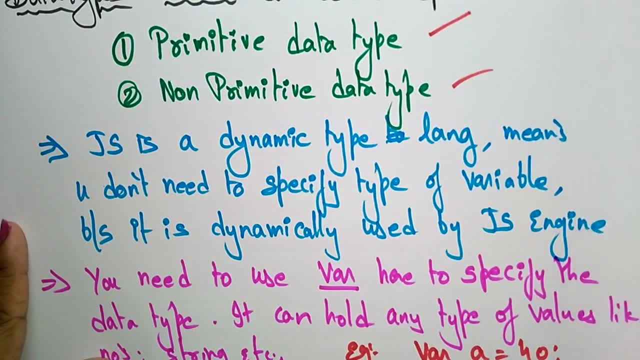 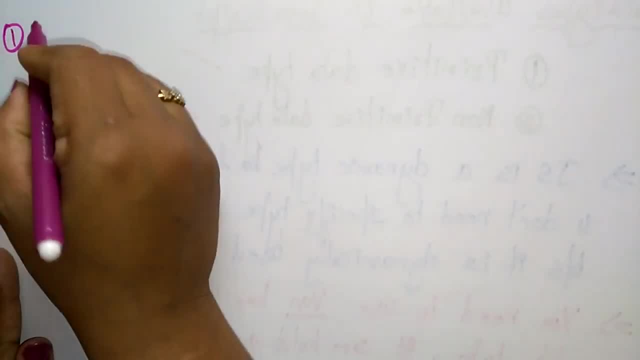 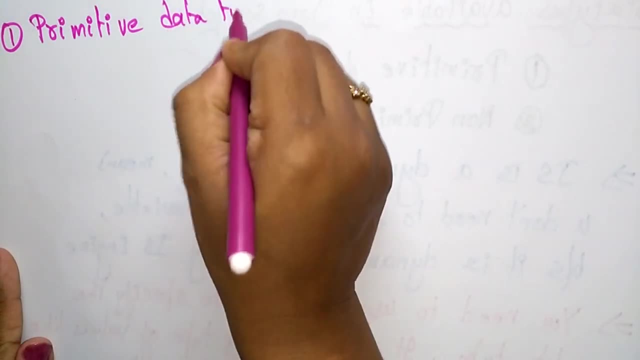 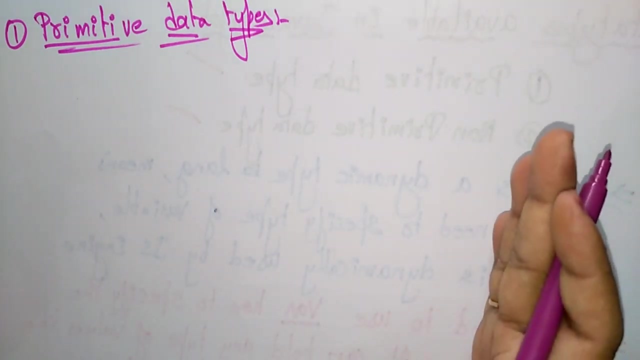 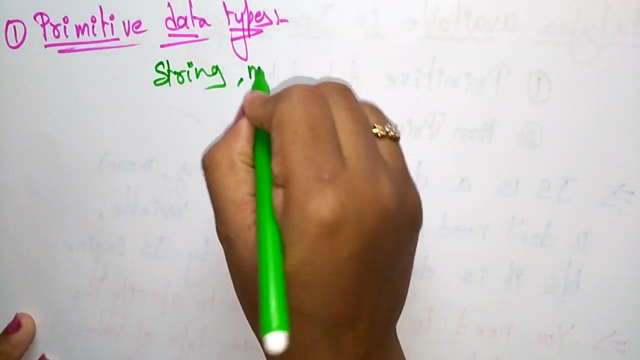 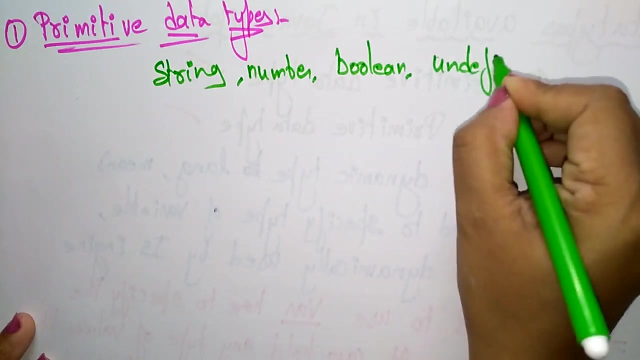 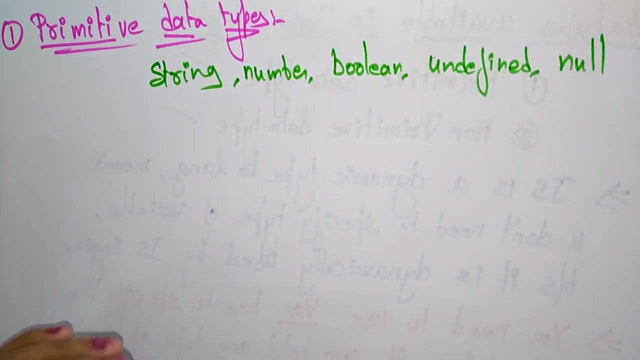 Now let's see what are the primitive data types and non-primitive data types. Let me write that Primitive data types. So there are five types of primitive data types. One is string, number, boolean, undefined and null. So these five are- you call it as a primitive data types. 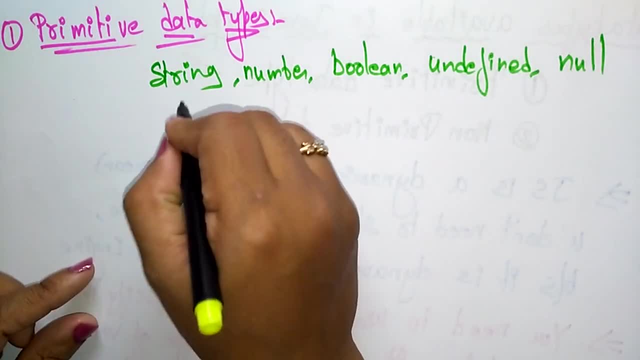 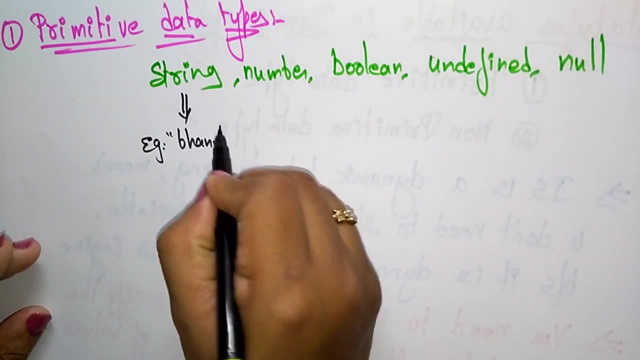 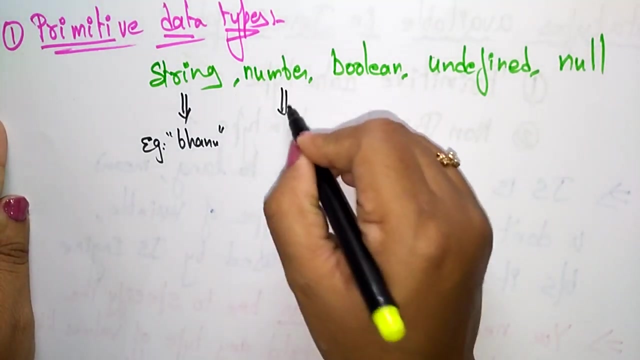 String is nothing but sequence of characters. You know that Sequence of characters, Like example, take the name, So it should be within the quotations. So string is a sequence of characters And number is a numeric values, So just a numeric value. 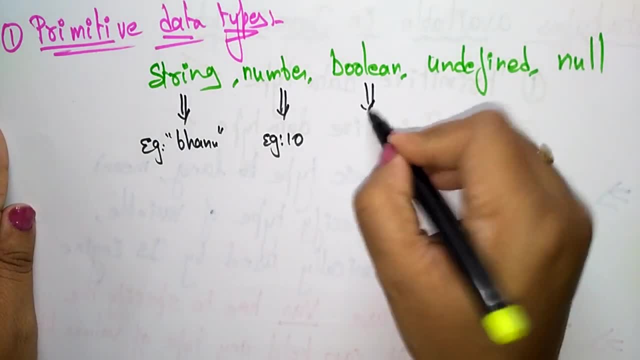 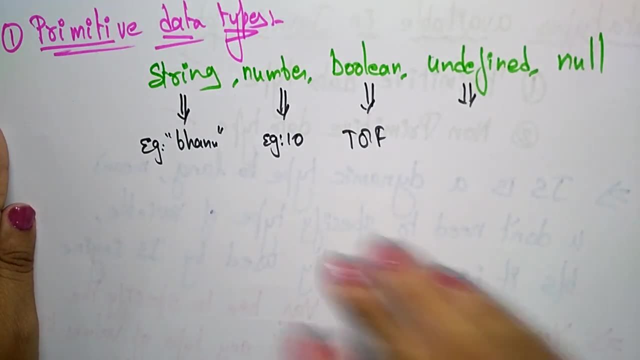 Just write a numeric value And the boolean is nothing. but it's a value, either true or a false. True or false, Then what about undefined, Undefined? Undefined, Undefined value means no value. You can't define that Undefined value. 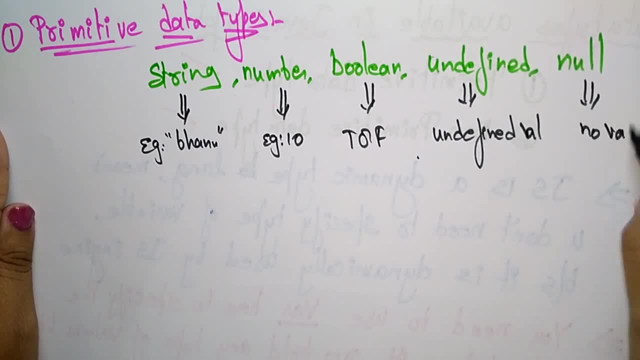 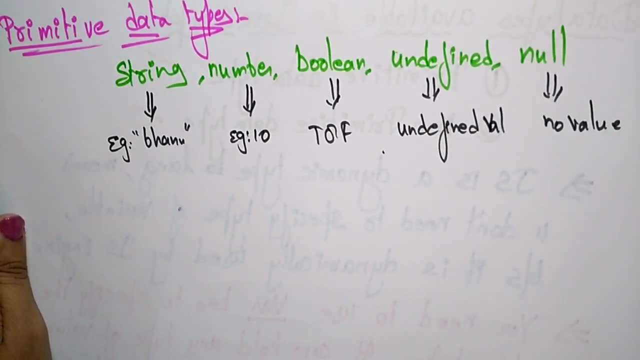 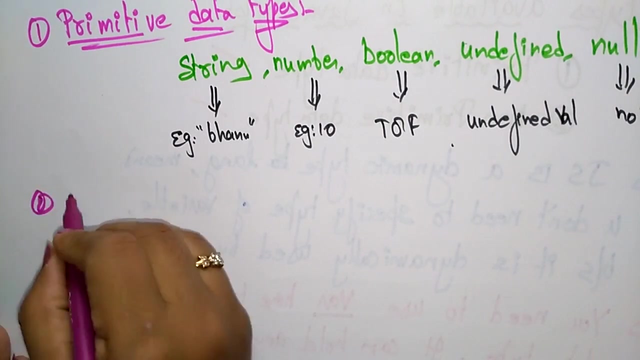 And the null means it's no value. So this is undefined. A value is there, but it is not defined. Undefined, And whereas null means no value, No value at all. So these are the five primitive data types. Now let's see the JavaScript. non-primitive data types. 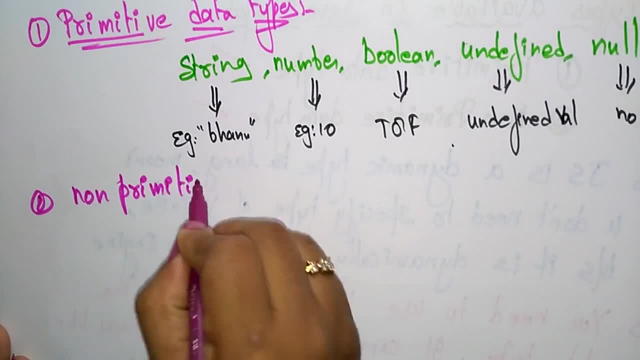 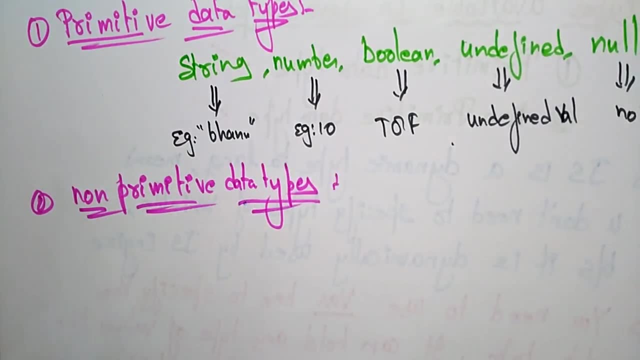 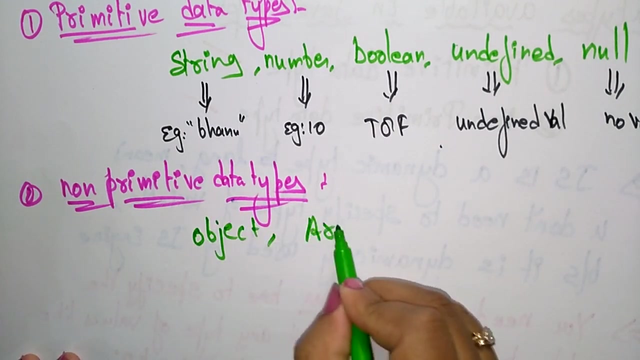 So the non-primitive data types are nothing but the objects, array and regular expression. So these are the three different non-primitive data types that are used in the JavaScript. Object means represents the instance through which the object is used. Object means represents the instance through which the object is used. 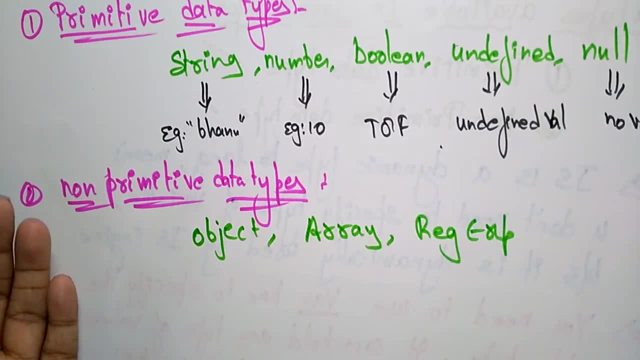 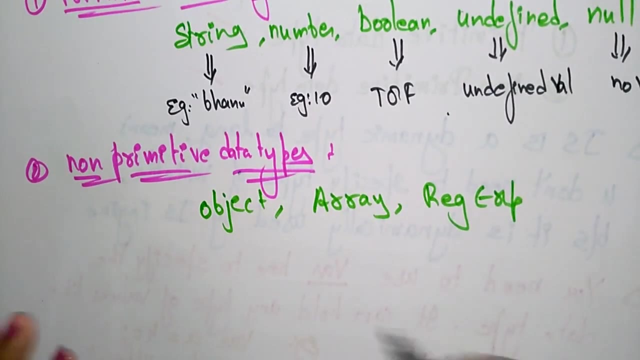 To which we can access, whatever it means: the members, the access, the members And whatever the array. Array is nothing but a group of similar values, and regular expression Represents is just an expression. So let me take a simple example to explain this: how you are going to use this primitive and non-primitive data types. 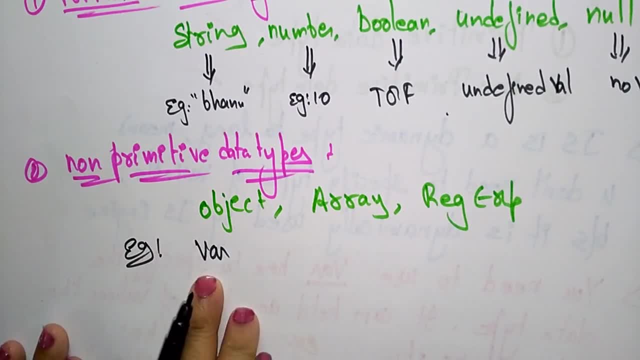 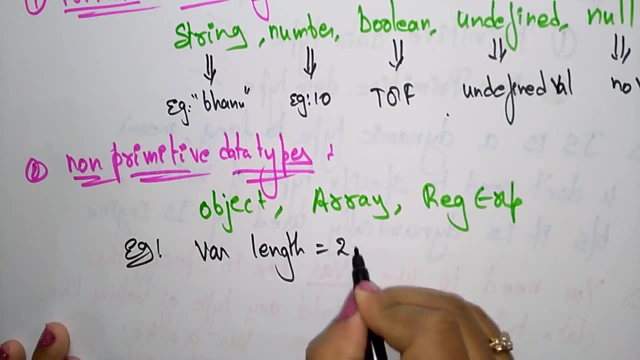 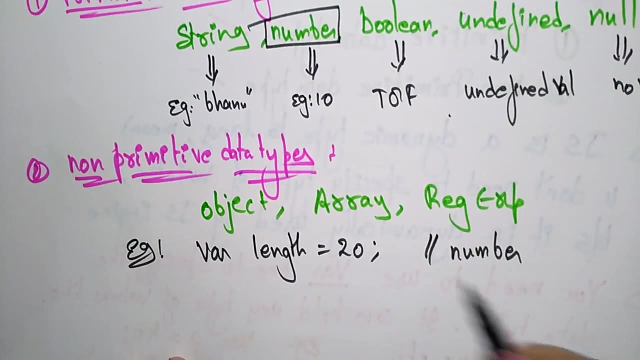 So whatever the value you want to be assigned, that should be assigned to the variable. So the variable is this: The variable is called variable length. Variable length is equal to 20.. So this is the number Means: primitive data type: Variable. let's take last name. 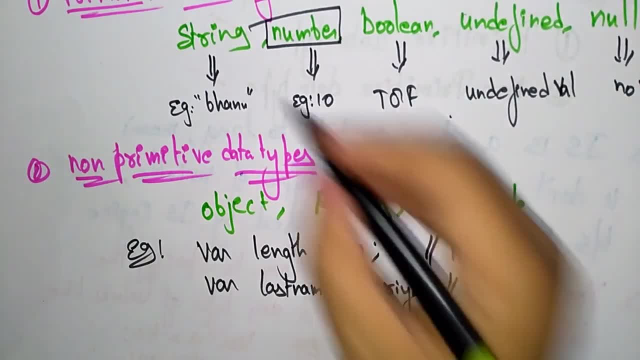 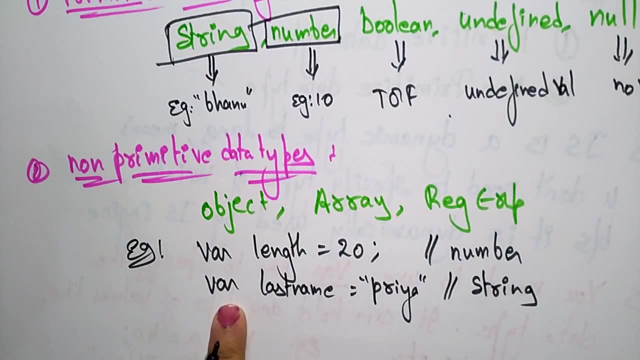 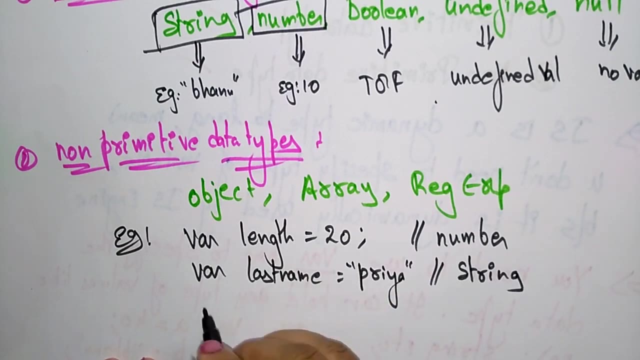 Priya. So this is a string. You can represent the string like this: Variable. so the variable is compulsory. Compulsory Variable: a name. whatever the name you want, to be right, you can write and assign the value. let's take variable x is equal to first name. 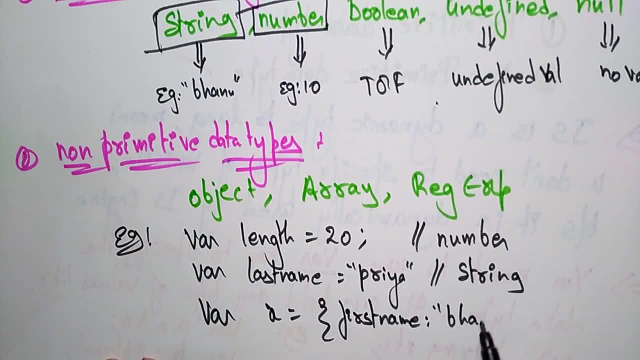 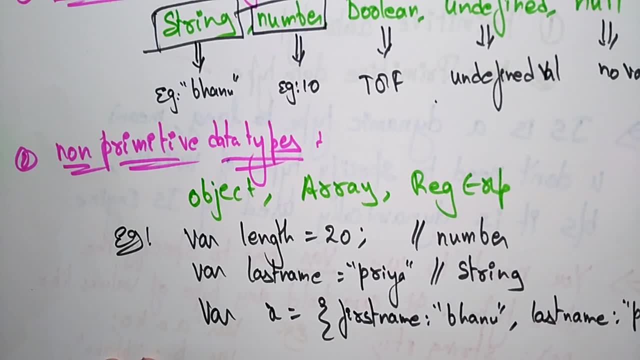 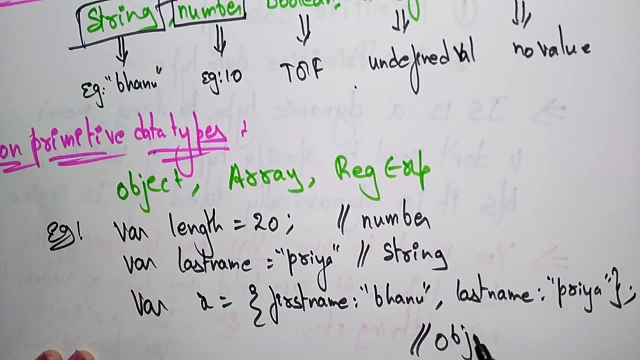 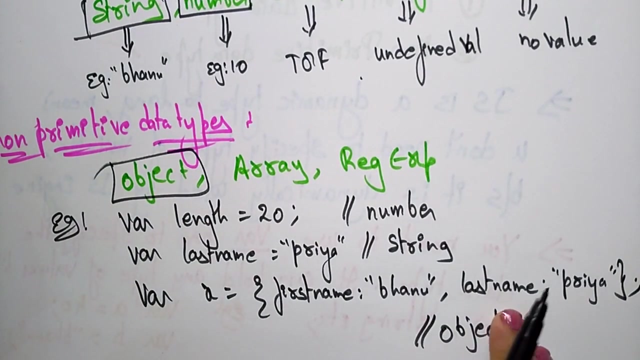 bhanu. last name: priya. just close it then. what type of representation is it? is the object. it's a non-primitive data type object. just calling the objects: the first name with bhanu and the last name is assigned to priya. so these are the different.